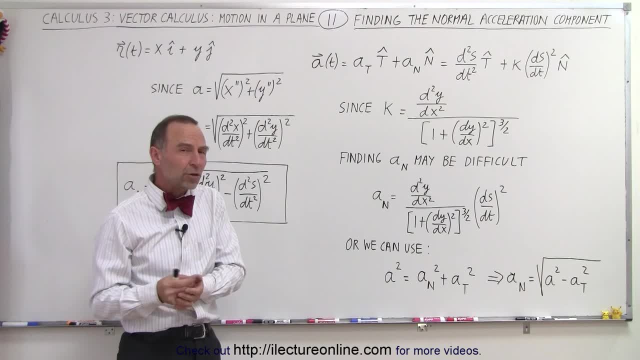 component of the acceleration. So instead we can use Pythagorean theorem. We realize that the magnitude of the acceleration is simply the slope of the acceleration. So instead we can use Pythagorean theorem. We realize that the magnitude of the acceleration is simply the slope of the 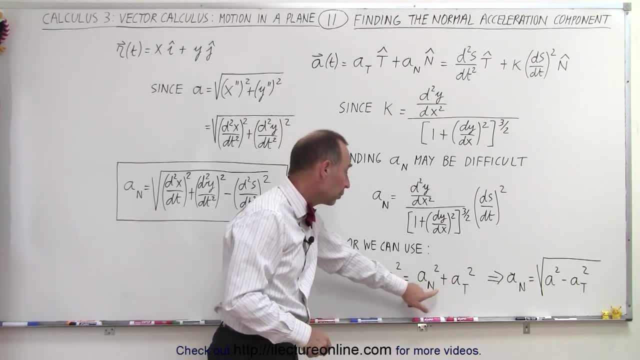 acceleration. So instead we can use Pythagorean theorem. We realize that the magnitude of the acceleration is simply the slope of the acceleration, So instead we can use Pythagorean theorem. We realize that the partial function of these two components is the difference between the normal component of 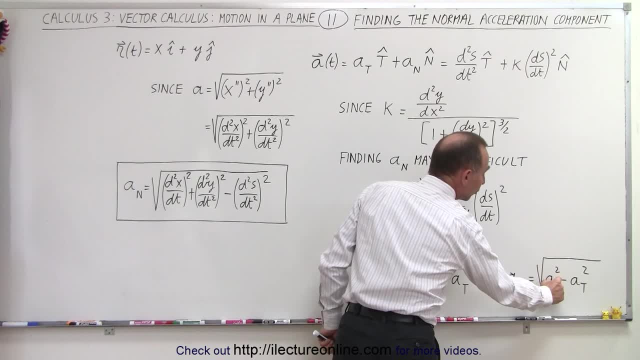 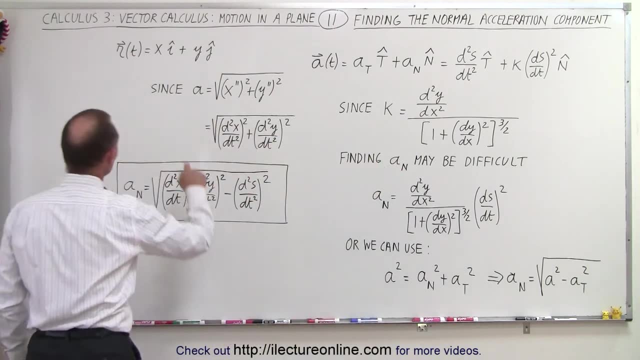 the acceleration and the value of the fitted equation, the tangentian component. Now, when we solve this equation for the normal plus that function calledグ, we're going to be having gross mosque and bowls down to the left. We're going to be having a constant where the주 is lower than the degree when we're talking about acceleration, and if we start 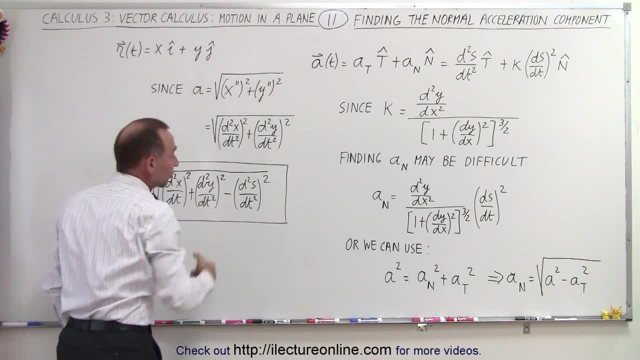 with a position vector which is x in the, the i-direction plus y in the and if we start with a position vector which is x in the i-direction plus y in the, x in the i-direction plus y in the, the Michigan kunzeστ Allen equation x, z, y, z and y. 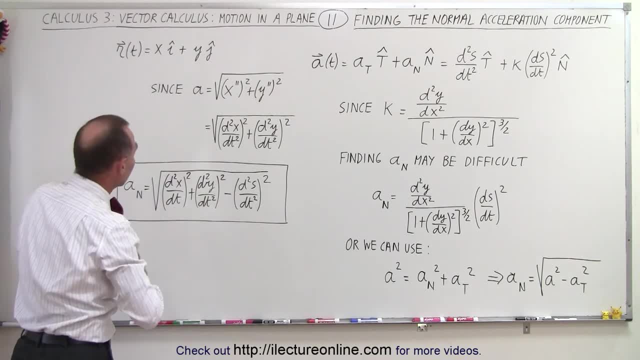 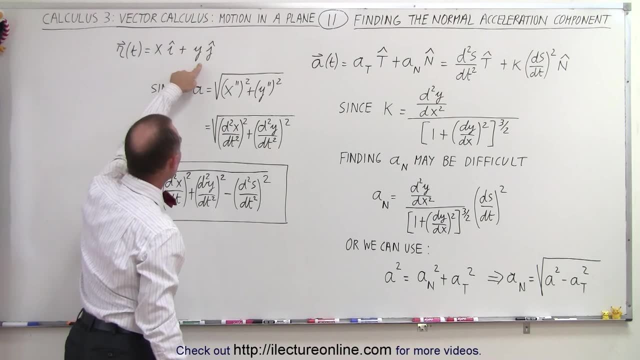 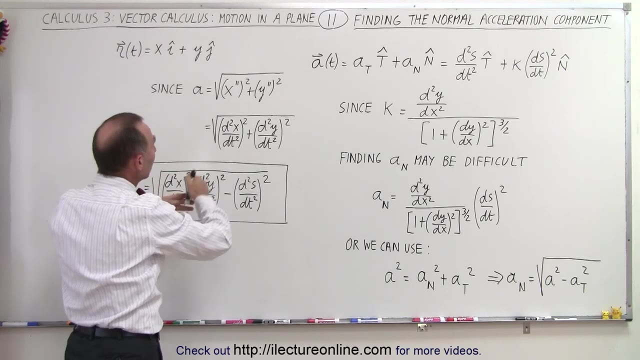 x and y, of course, being functions of the parametric variable time, Then the acceleration can be found by taking the second derivative of an x component, the second derivative of the y component, and then we square both components, add them together, take the square root, and that gives us the magnitude of the total acceleration vector. 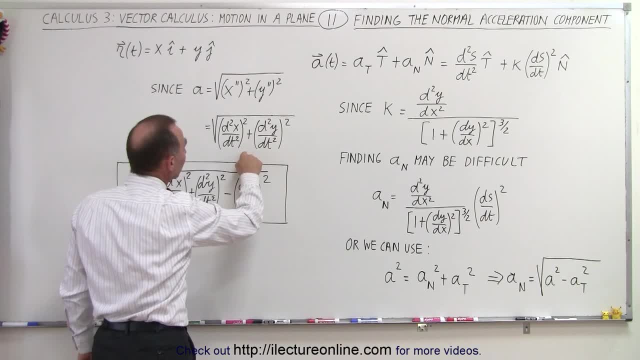 And of course that's expressed in terms of the x and the y components of the acceleration. So x double prime is d square, x, dt squared. y double prime is d square, y, dt squared. We take those two, we square them, we add them together. take the square root. 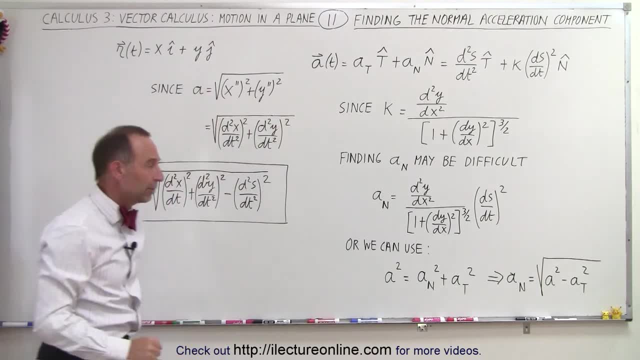 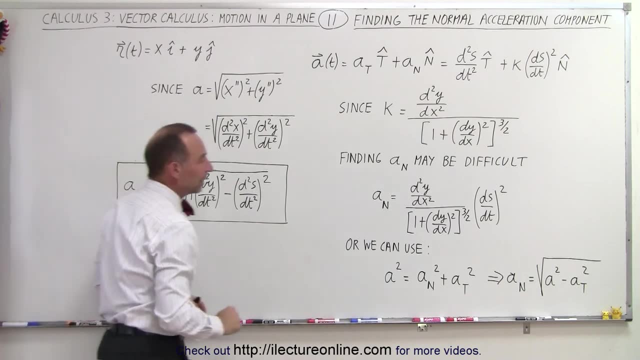 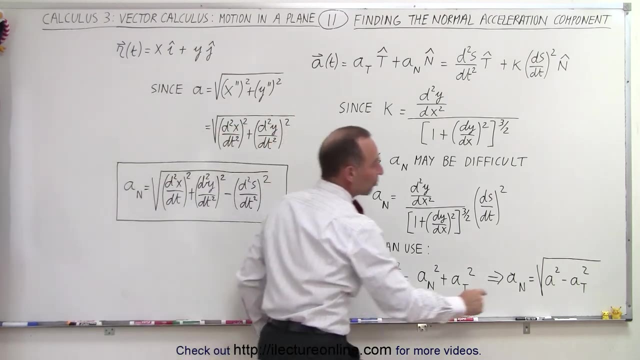 that's the magnitude of the acceleration vector. Of course. if we then square that magnitude, the square root symbol goes away. but now, when we find a sub m that is equal to the square root of the, a squared. a squared is right here, minus the tangential component: squared. 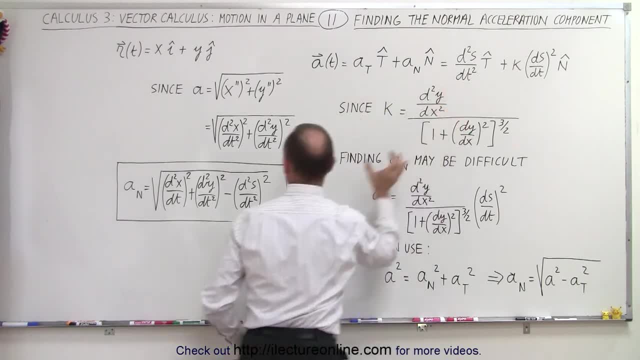 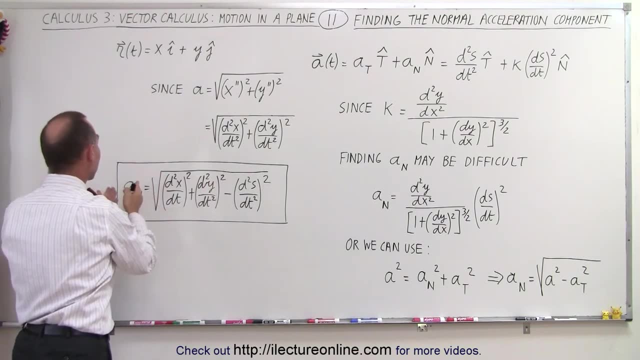 Now that's a squared. The tangential component right here is this quantity. so we take that quantity and we square it as well, and subtract it from the total magnitude of the acceleration. take the square root of that. that gives us the normal component of the acceleration. 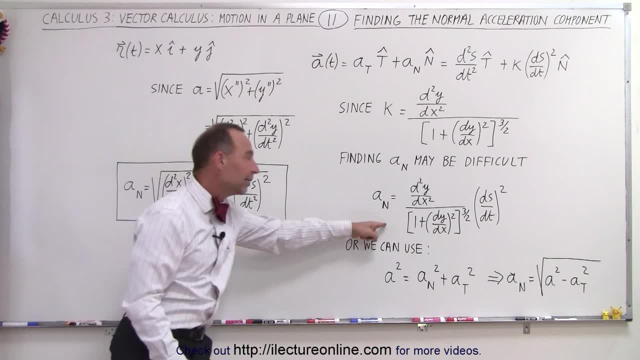 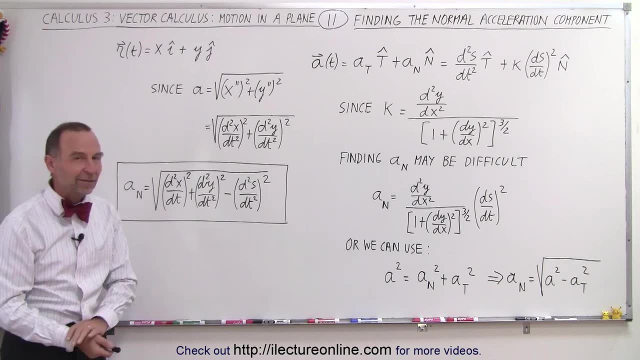 And this method is quite often easier to use than this method, at least. Now. you have two methods. either one will give you the answer, but sometimes I prefer this one. it makes it easier and that's how it's done. Here's an example of an incompetent method. and you can also take the right part of the equation and add it to this. Now you can see here that you have a percent18, and now that equation can also be set to scale. So what are these two Chinese cake firstþs that we have here? and once we have the result for times we follow it back in to the straight asked equation.